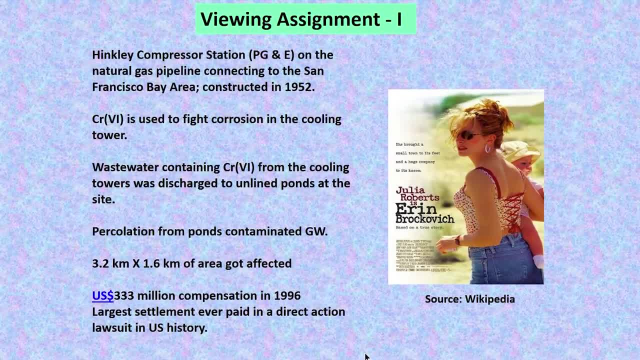 was being discharged into an unlined ponds at the site. This was a while ago And since this is an unlined pond, the percolation from ponds eventually reached the groundwater and it contaminated. It contaminated an area of 3.2 kilometers by 1.6 kilometers and because of that, 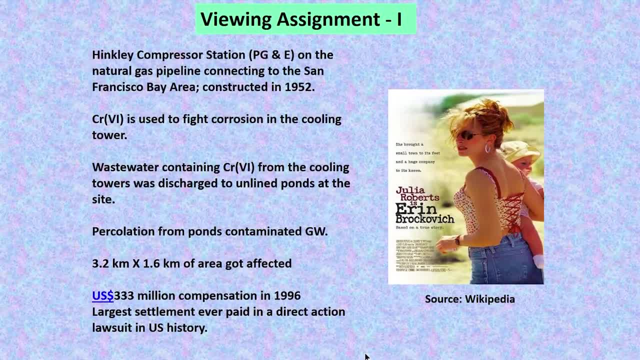 contamination. lot of other problems arose and there was a lawsuit and dollar 333 million dollars compensation was given in 1996 and this is the largest settlement ever paid in a direct action lawsuit in the history of United States. So there is a movie about this and I would suggest. 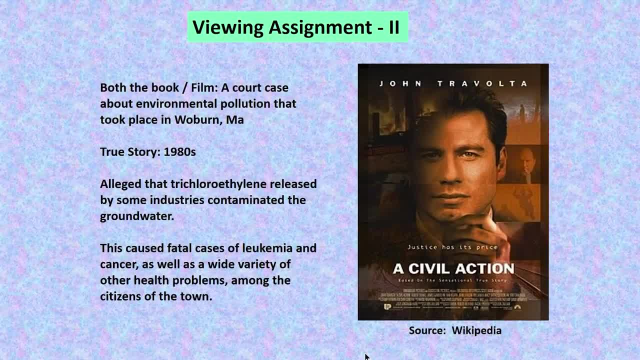 that you watch this movie. There is another movie called a Civil Action starring John Travolta, and it is based on a book by the same title, Civil Action. There was a court case about environmental pollution that took place in Auburn, Massachusetts. This was a true story that 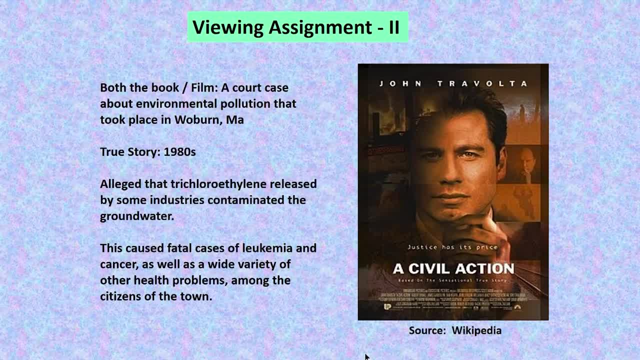 happened in 1980s. It was alleged that trichloroethylene released by some industries contaminated the groundwater. And the reason for the contamination of the groundwater? it was because the and this caused fatal cases of Leukemia and cancer, as well as a wide variety of other. 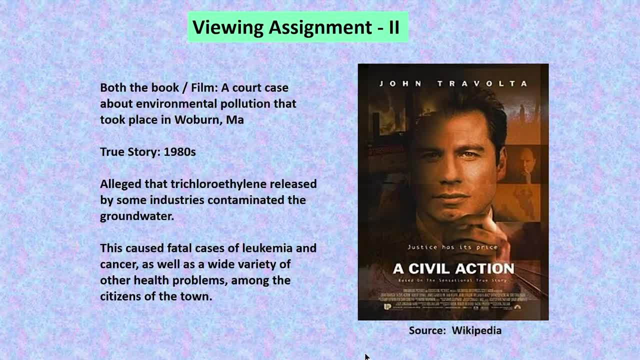 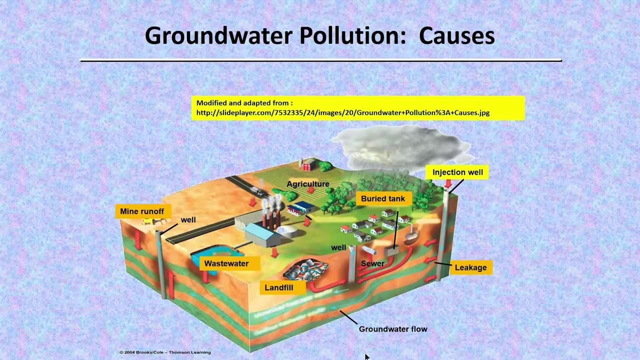 health problems among the citizens of the town. so there was a court case. I suggest that you watch both these movies. okay, Now, groundwater pollution. what are the causes? We have lot of landfills and the landfill, the leachate from the landfill and if the 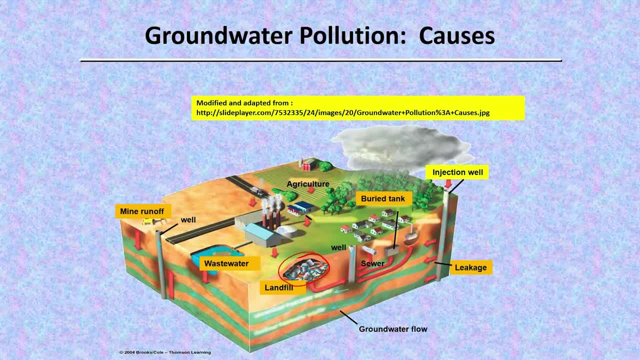 liners are not working properly, or if the liners are not provided, then the leachate from the landfill will go down and then can contaminate any of your aquifers. This is what we call an unconfined landfill. That is the water table I mean. the water here is exposed to atmospheric pressure, so 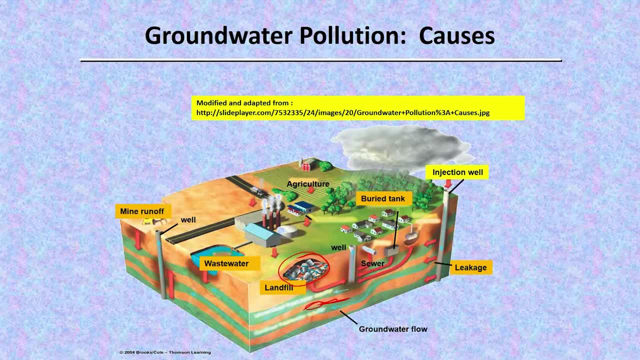 this is an unconfined aquifer, whereas this part here is what we call a confined aquifer. It has a confining layer below as well as confining layer above, So this landfill leachate can go and then contaminate your unconfined aquifer. 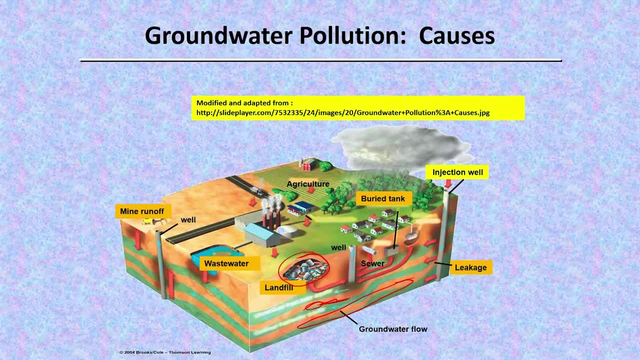 Okay, We may be taking water from this unconfined aquifer through wells for drinking or some other purpose so that well water could be contaminated. It is not only the landfills, but we may have buried tanks which may be carrying hazardous chemicals and if there is a leakage from these buried tanks, the leakage of these hazardous 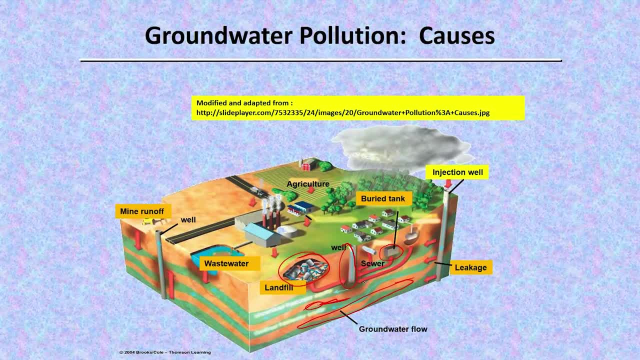 chemicals, They can also contaminate our unconfined aquifer. Then we have industries and waste water from these industries- if it is stored in waste water lagoons or waste water ponds, and the leachate from this waste water ponds or waste. 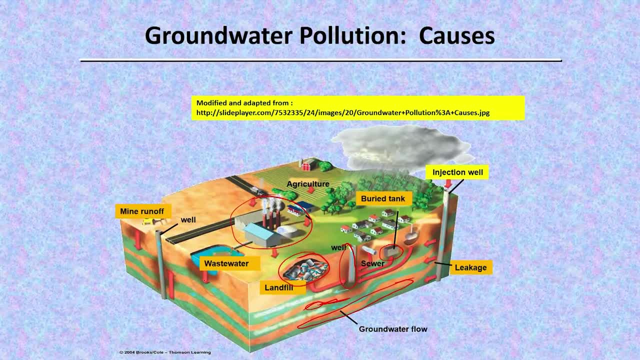 water lagoons can also move down through the soil and then can contaminate this unconfined aquifer. We may have injection wells through which we may be injecting either partially treated waste water or untreated waste water for ground water storage into very, very deep aquifers. 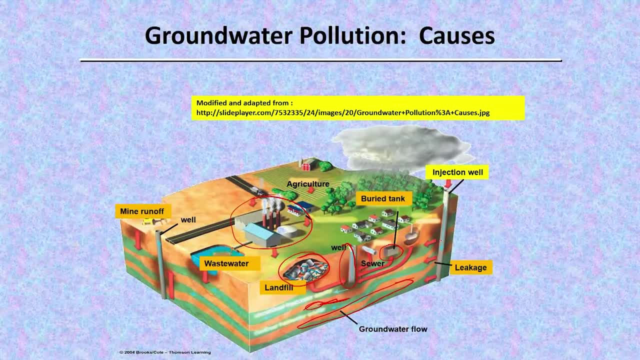 and the casing of these injection wells could be leaking and that may leak into even your unconfined aquifer, very deep confined aquifers. Aquifers are water bearing stratum. okay, in the underground and your ground water can be contaminated or you may have a mine runoff. also, if it is not managed properly, it can. 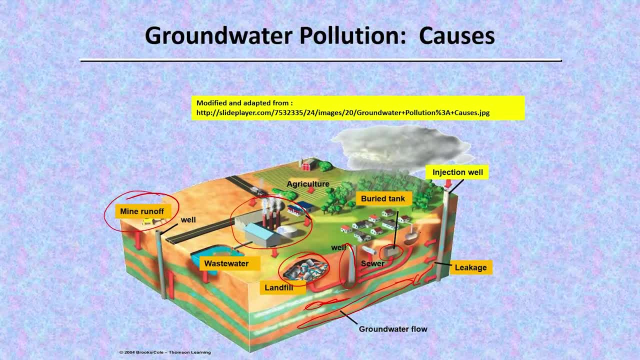 contaminate the ground water and we have septic tanks from the households. we have septic tanks. The septic tanks are not functioning properly. the leakage or the leachate from the septic tanks can also pollute your ground water and one more important source for the pollution. 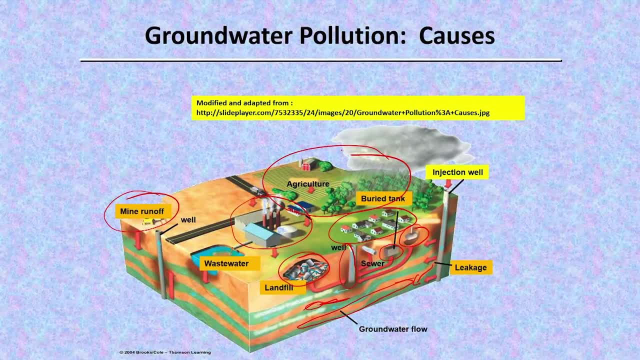 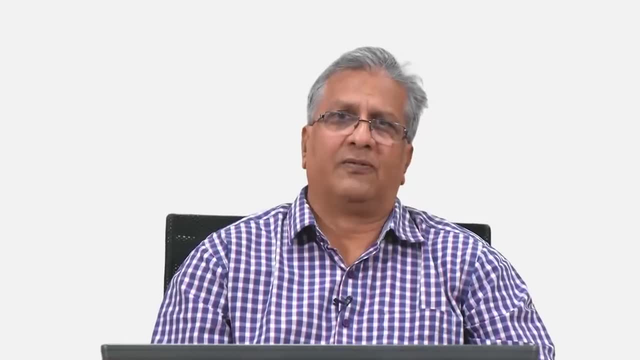 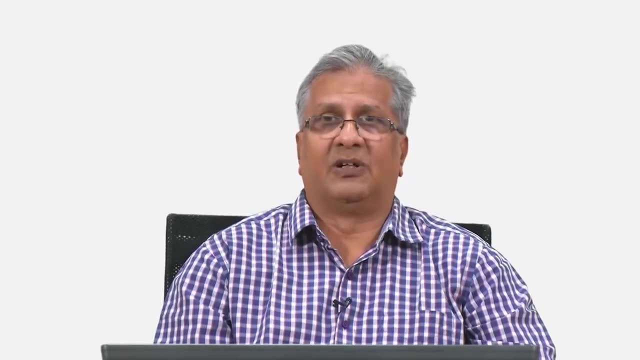 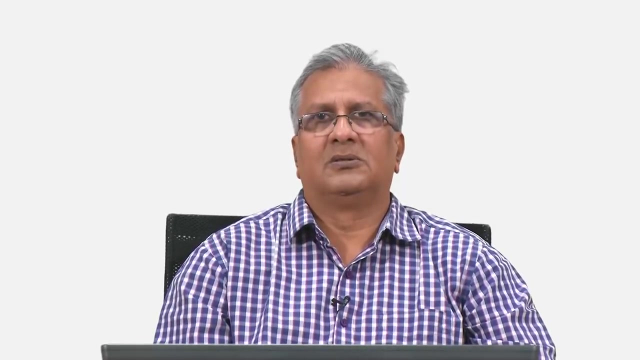 of ground water is the agricultural activities For increasing the food production and for protecting the crops. we may be using lot of fertilizers and pesticides which are nothing but chemicals, And some of them are very bad for human health. and if you use these pesticides and fertilizers, 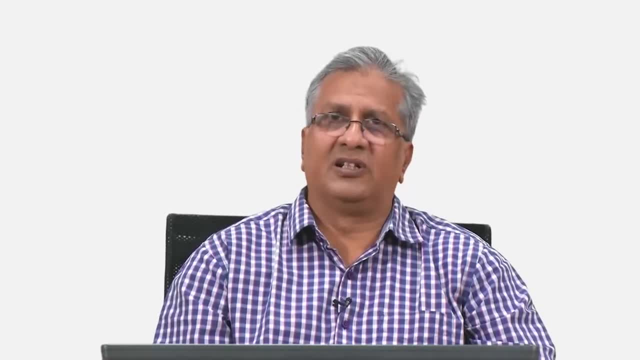 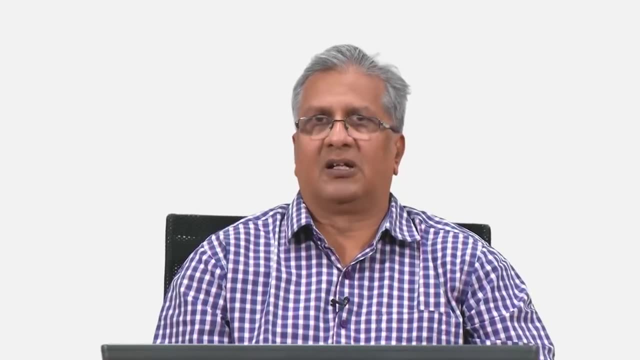 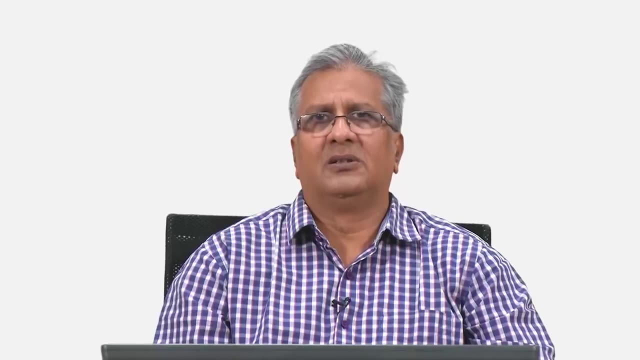 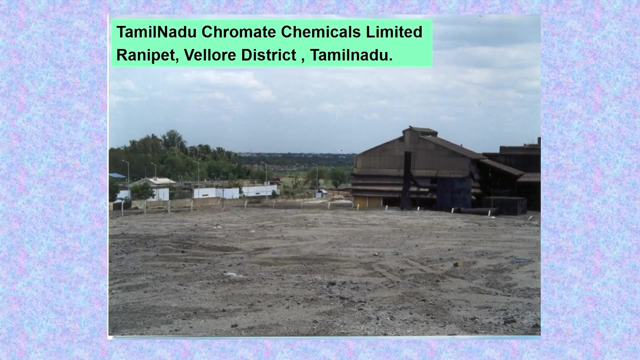 without any control, without any proper attention, then, along with the irrigation water or the rain water, these things can leach into the ground and then contaminate the ground water. So there are several causes for this ground water pollution. Well, first we have the 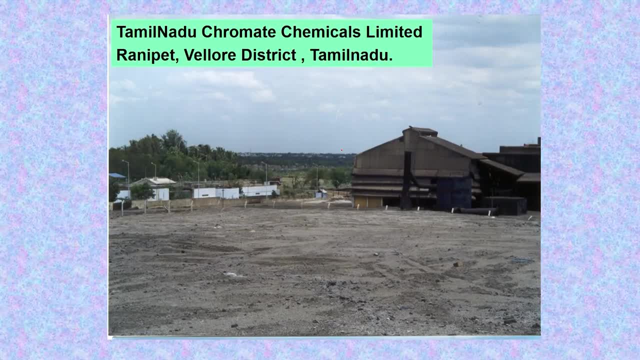 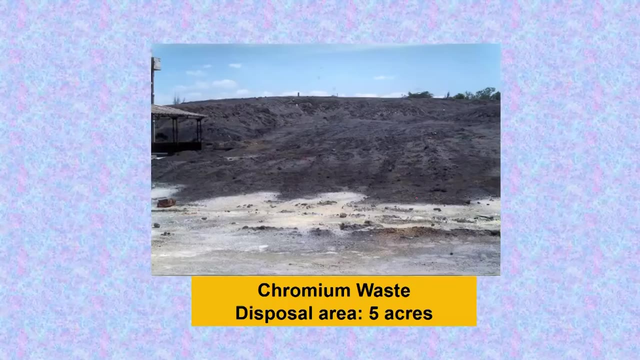 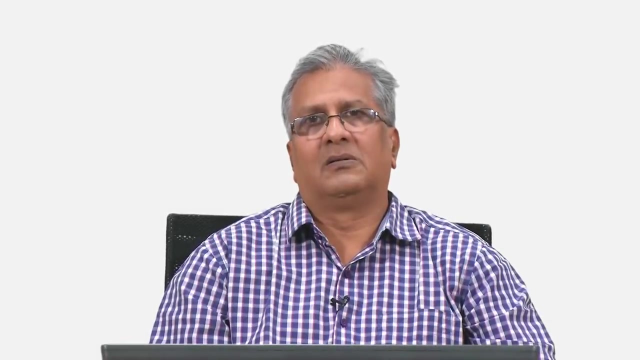 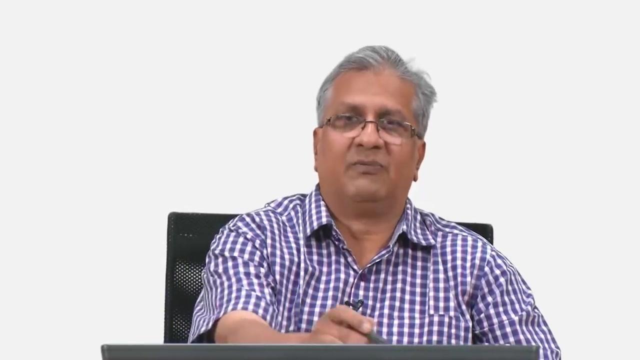 1. 受, then then take their 2. へ. there was a case in the lassen, the Burma. proper attention: The chromium waste, the disposal area is still there. it is about 5 acres of land over which this chromium waste is disposed, and it is open to the rains, and so whenever 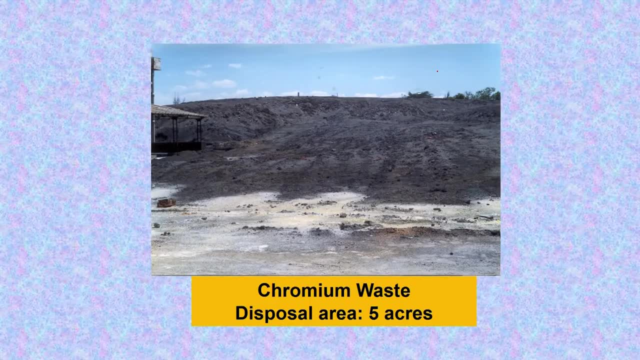 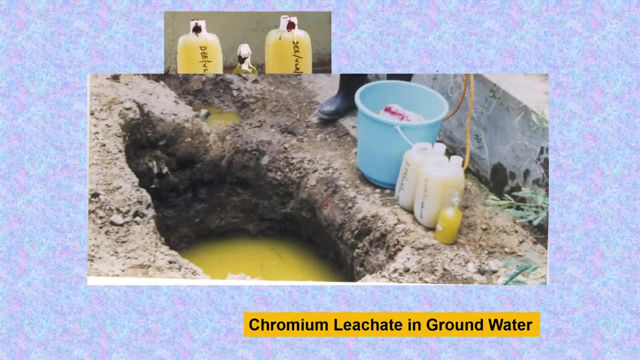 there is a rain, then hexavalent chromium gets leached into the rain water and this rain water is infiltrating into the ground and you can see the groundwater is contaminated with chromium leachate. So you can see the groundwater which is in yellow color. this 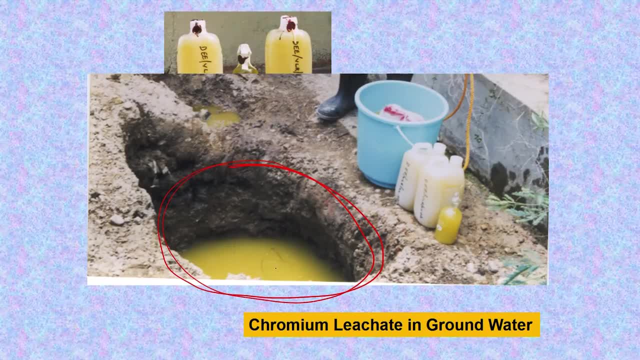 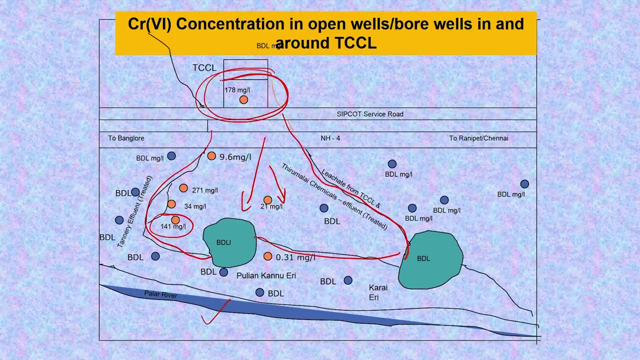 is completely contaminated with chromium leachate and once it gets and it reaches the groundwater table, it just does not stay there. It starts moving along with the groundwater. for example, this is the location of the dump site where one of my colleagues has gone and 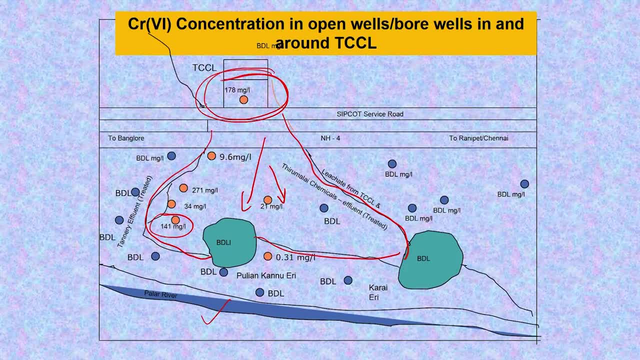 then measured the concentrations in the groundwater. it is 178 milligrams per litre there, And Professor Liji Philip, my colleague, who measured groundwater levels along with her colleagues in other locations, also has drawn this plume shape, And here it is around 141 milligrams per litre. and it is not just staying there. it cannot. 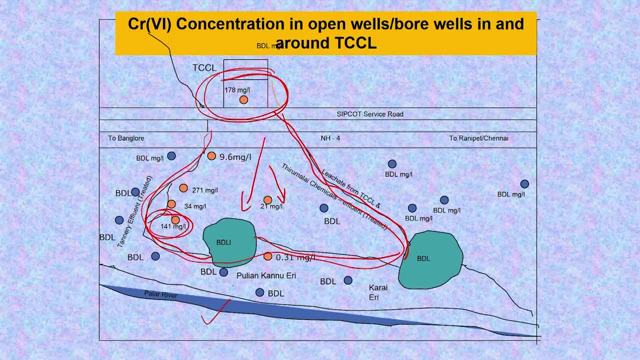 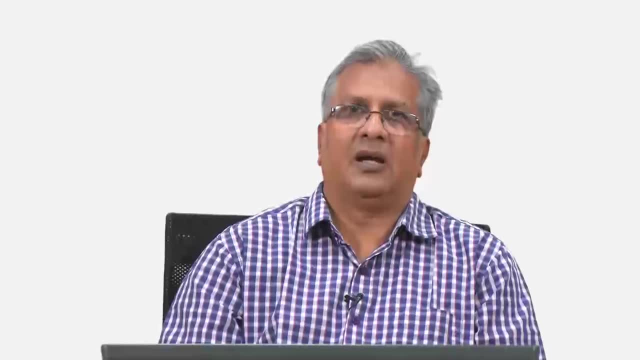 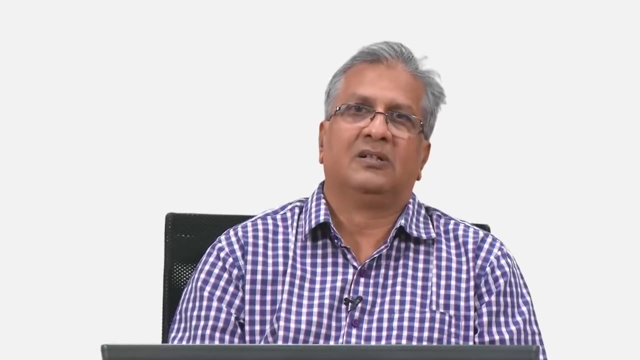 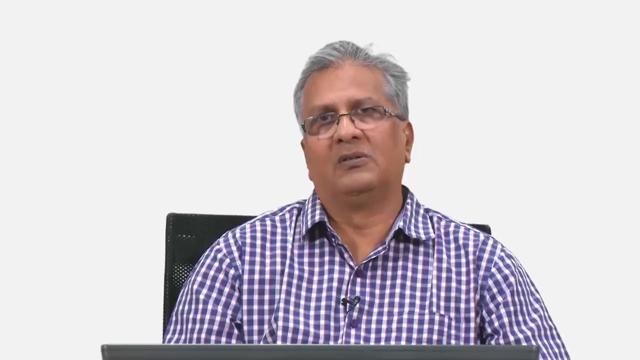 just stay there. it starts moving, and it starts moving towards the lower water levels and then we have a Pala river and it has a lot of good groundwater. Once this plume reaches this Pala river, then that groundwater also will get contaminated. So we have to be careful while we are disposing the sludge, and then we also have to think. 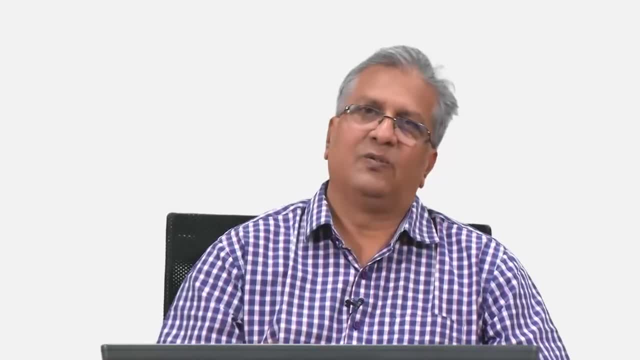 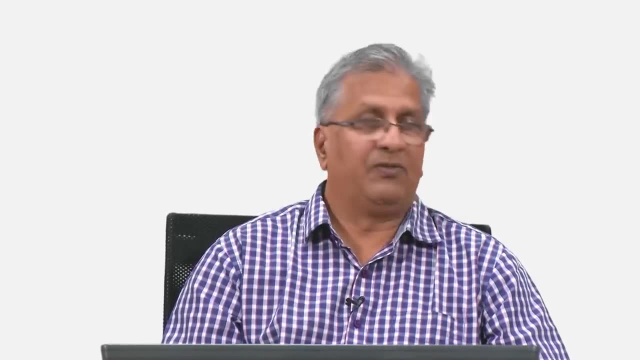 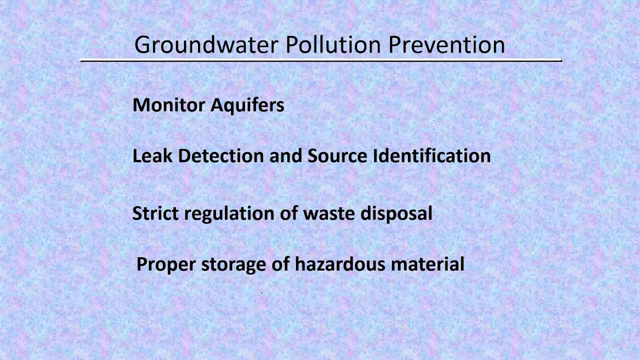 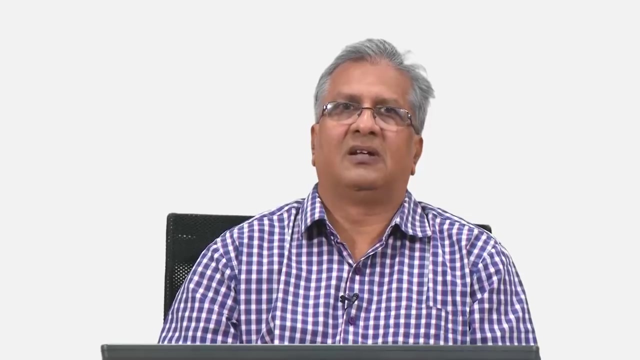 about? what are the ways by which we can treat this groundwater so that this groundwater can be used in future? What are the different ways of preventing the groundwater pollution? First and foremost thing, we need to monitor the aquifers. that means we have to take the water samples at frequent intervals and then analyse this water. 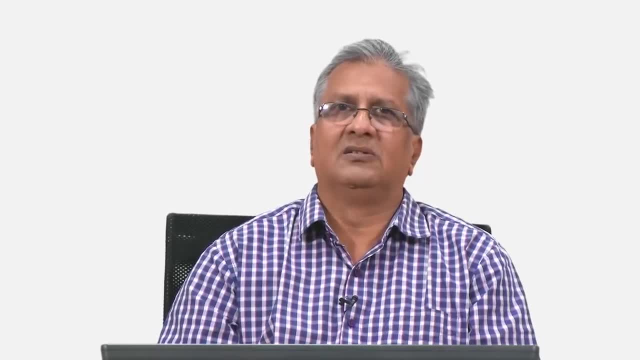 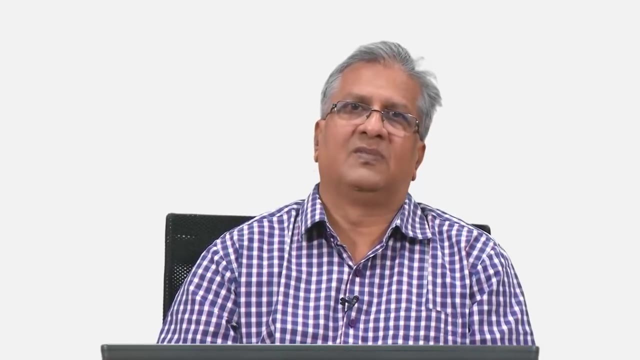 samples for any possible contamination. So we have to monitor aquifers so that we would know What is the level of contamination and how far the plume has moved. the contaminant, contamination has moved. What is its transport? What is the fate of this contaminant? For all that, 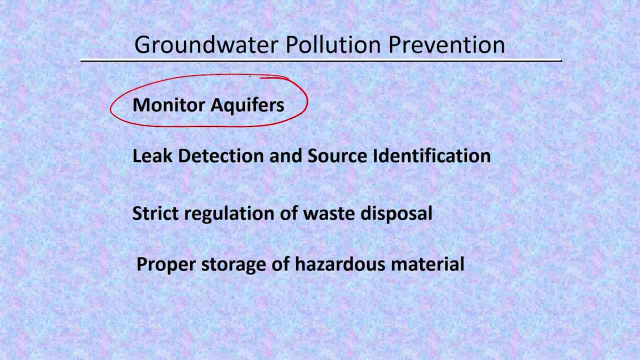 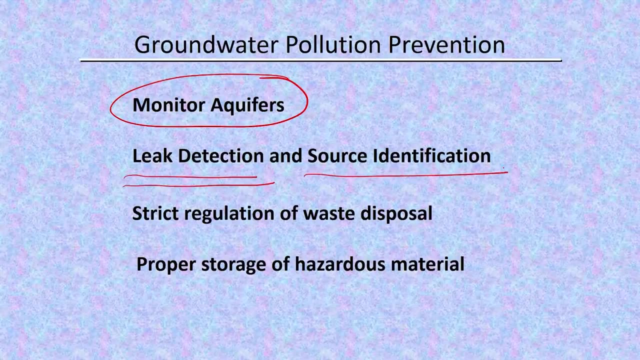 we need to monitor the aquifers, Then we also have to worry about which are the places where the leaks are occurring or the spills are occurring. So we have to have a leak detection system and a source identification or environmental forensics is also very important Once we detect. 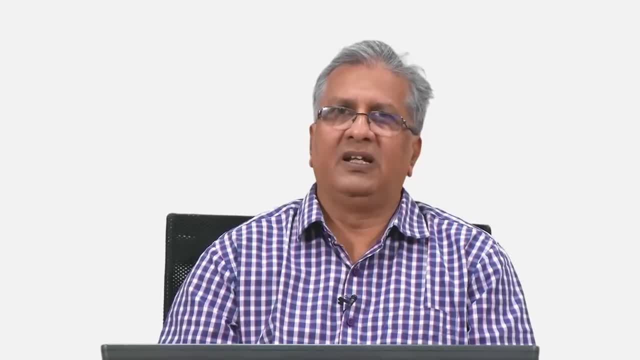 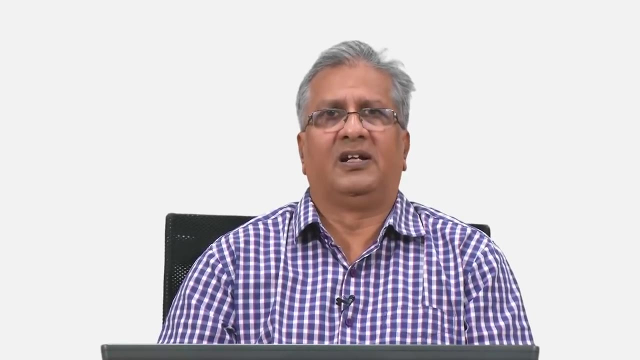 that groundwater got polluted, we need to find out where this pollution is coming from. So the source identification is very important and it is not also very easy, but it is very important. in terms of groundwater quality management, We need to put very strict regulation. 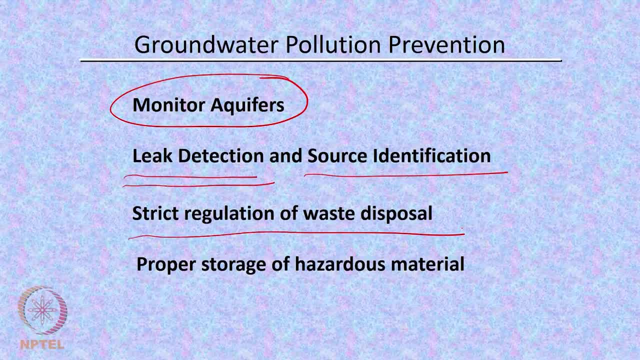 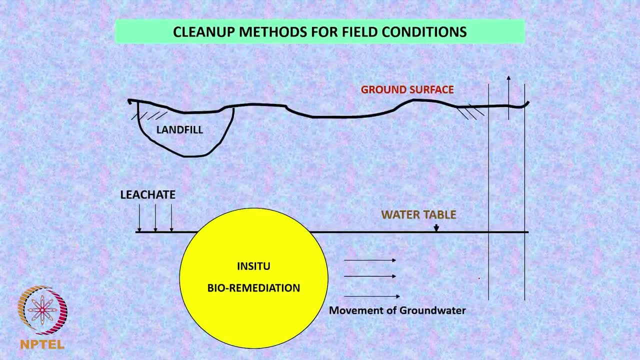 regulations on waste disposal and we need to have proper storage of hazardous material. One of the ways by which we can treat the contaminated groundwater is what we call pump and treat, That is, you pump out the water from the ground and then you send it back to. 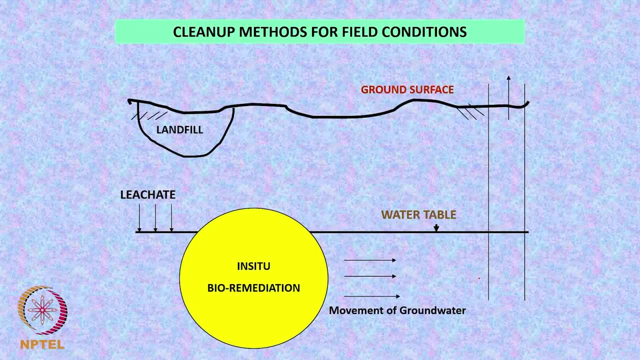 the source And then you get a secondary pump and a secondary treatment And then you send it back to the source And then you câll, pump and treat to save that funding. In other words, you pump that water through proper treatment plants and design the treatment plants according. 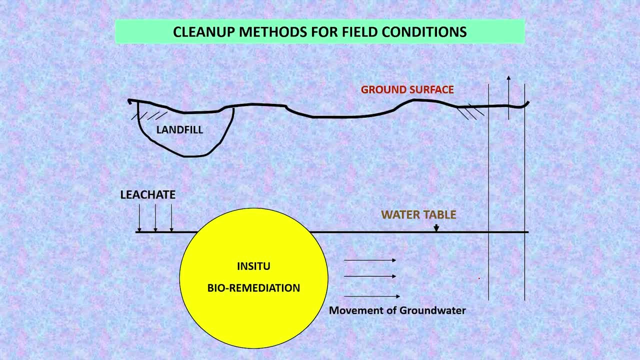 to what kind of a contaminants we have. We can use either biological methods or chemical methods for treating this contaminated groundwater in the treatment plants and then put that treated groundwater back into aquifer through what we call recharge wells. This is what we term as pump and treat methods. 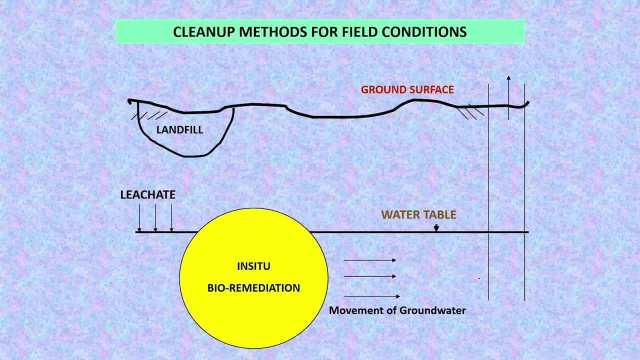 But we can also have in situ treatment. that is what schematically shown here in this picture. Let us say we have a landfill here and this landfill is leaking And the leachate from the landfill has come to the aquifer and there is a pumping. well, 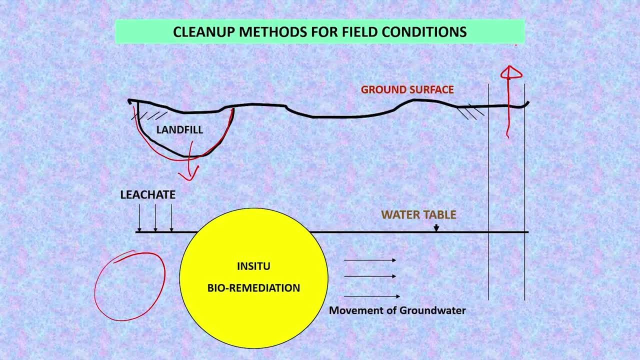 here, which is pumping the water for some beneficial purpose, And because it is pumping, the groundwater will flow in this direction. As the groundwater is going in this direction, the contaminant Also moves along. with this leachate which has come here, it will also start moving into. 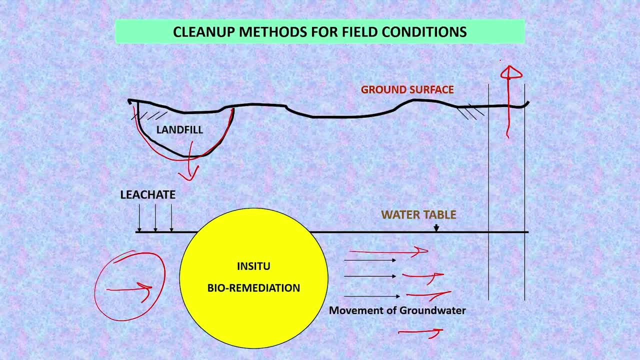 the well and eventually we get contaminated water from this well. So what we can do is, between this location here and this well, we can have what we call an in situ bioremediation. We can introduce a very special bacteria like chromium, reducing bacteria. 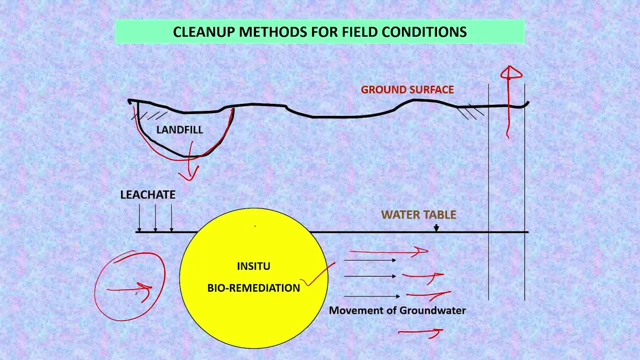 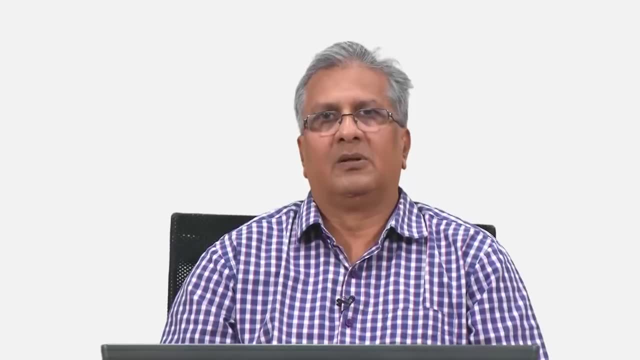 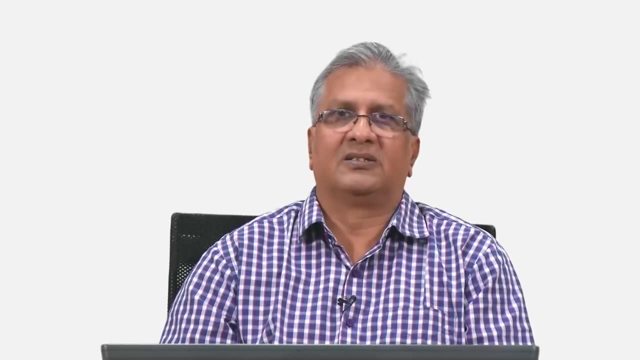 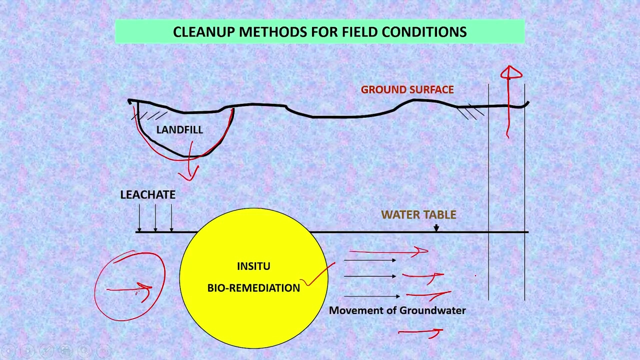 In this location and this chromium reducing bacteria can convert hexavalent chromium to trivalent chromium, whose solubility is less, And then it will precipitate out and it will get fixed on to the solids. So, whatever the water that comes towards the downstream side will be free of hexavalent. 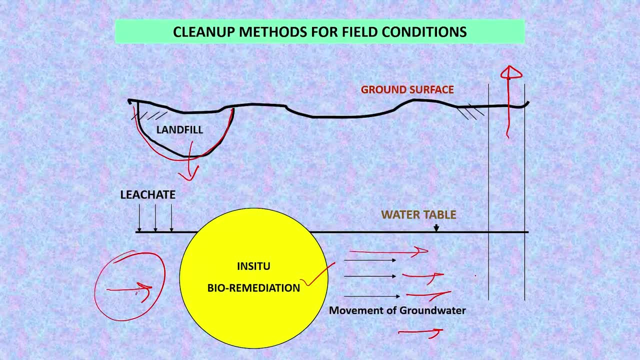 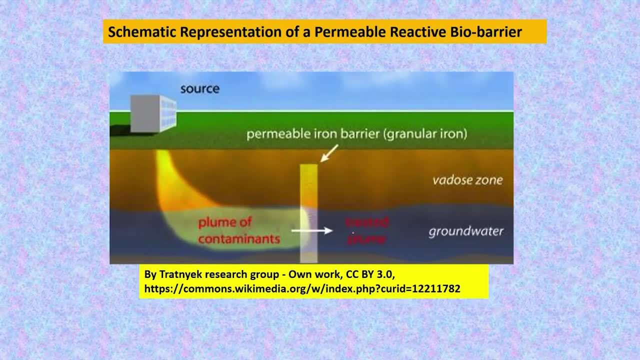 chromium. So this is what we call an in situ bioremediation technique, And for this we can have permeable reactive bio barriers or permeable reactive barriers. Here this is a barrier where we have introduced the appropriate chemicals or bacteria And as the plume is moving towards this direction and it moves through this permeable barrier, 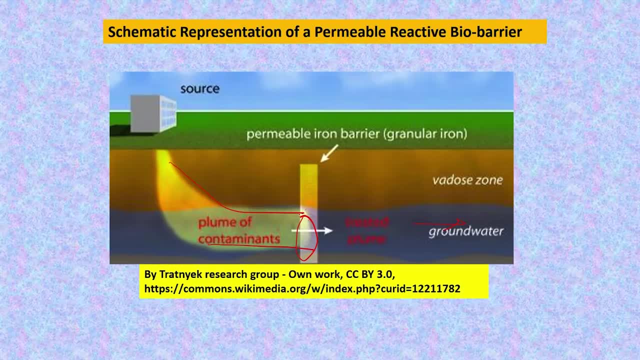 So these reactions will occur in this permeable barrier and then either the contaminant is degraded or contaminant is transformed to less harmful substances, like in case of hexavalent chromium. there is a bio. you can use bio transformation to trivalent chromium and then clean water. 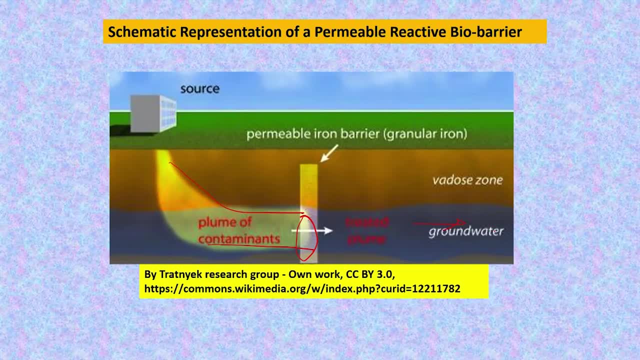 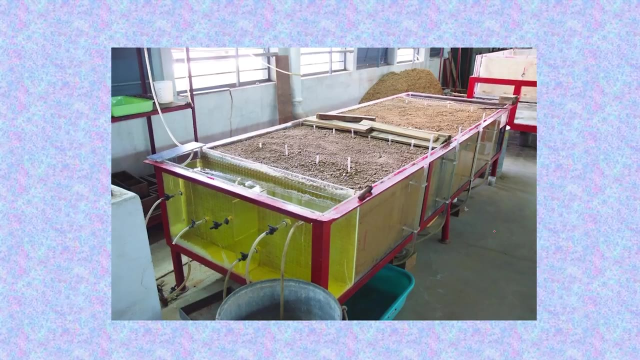 comes out on this side So we can have chromium reducing in the ground along with the groundwater towards the downstream side. and here she put a permeable barrier and introduced the chromium reducing bacteria that she and her colleagues have isolated and enriched, And this chromium reducing bacteria converts. 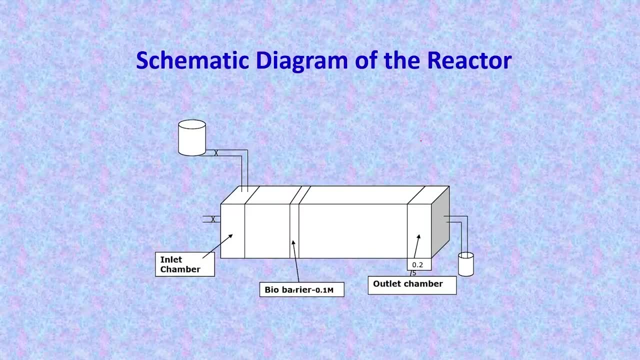 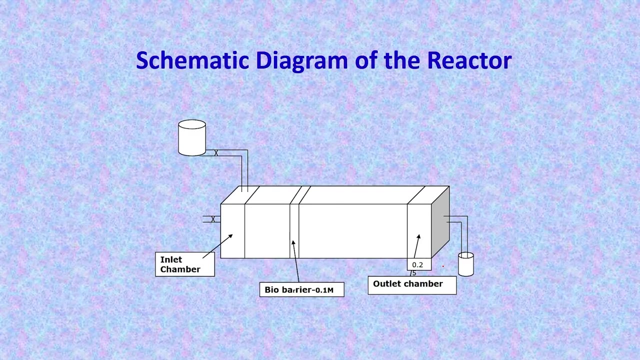 CR 6 to CR 3.. This is the schematic diagram. is an inlet chamber. here there is a bio barrier. it is only 10 centimetres thick. this total length is about 3 metres and there is an outlet chamber. 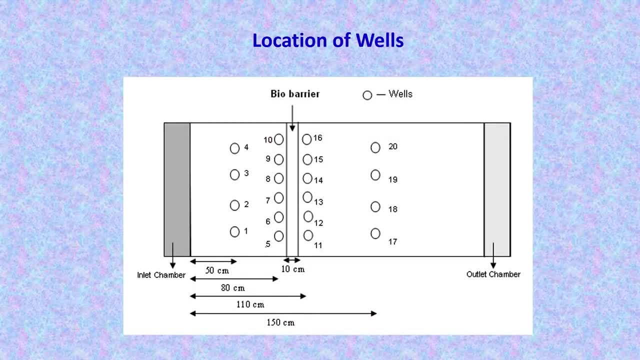 and then we have lot of these monitoring wells: 1,, 2,, 3,, 4,, 2,, 10 monitoring wells on the upstream side of the bio barrier and then 16 to I mean 11 to 20- the monitoring wells. 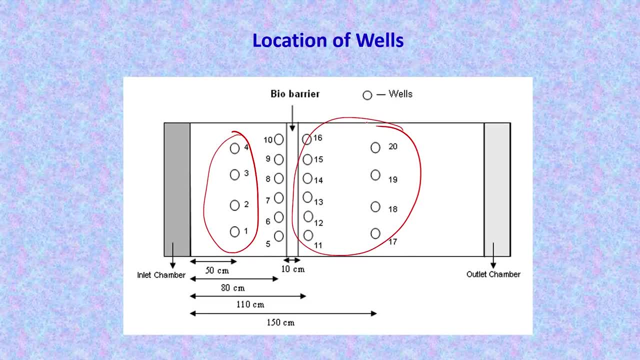 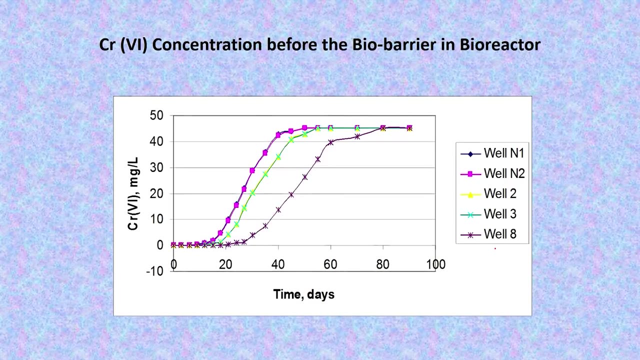 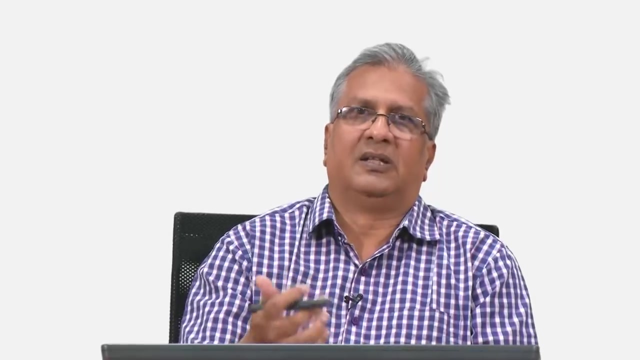 on the downstream side, We had taken samples from these monitoring wells and then analysed for the presence of hexavalent chromium, or what is its concentration, and experiments have shown that upstream of the bio barrier, There was an eventual breakthrough of the hexavalent chromium has reached these monitoring. 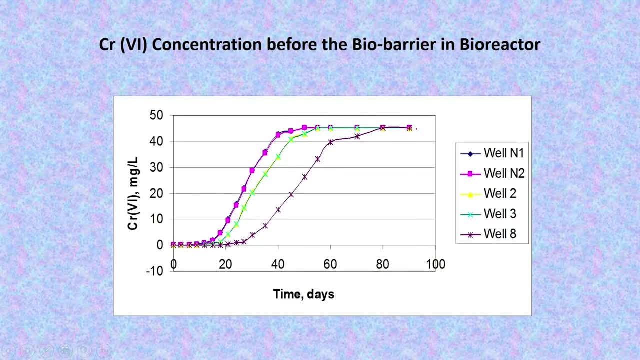 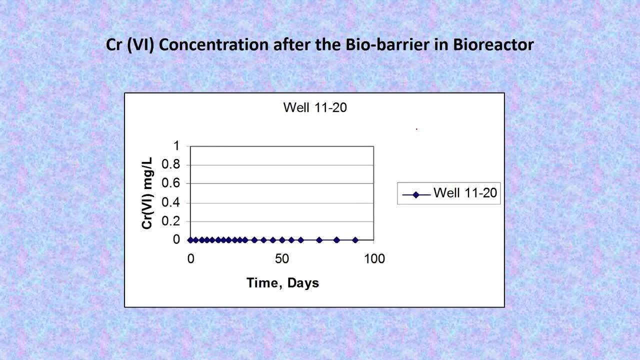 wells and the concentration was as high as 45 milligrams per litre, whereas on the downstream side in the wells 11 to 20, there is no hexavalent chromium. That means all the hexavalent chromium got converted to trivalent chromium In the bio barrier. this is just an example of how one can do in-situ treatment of polluted 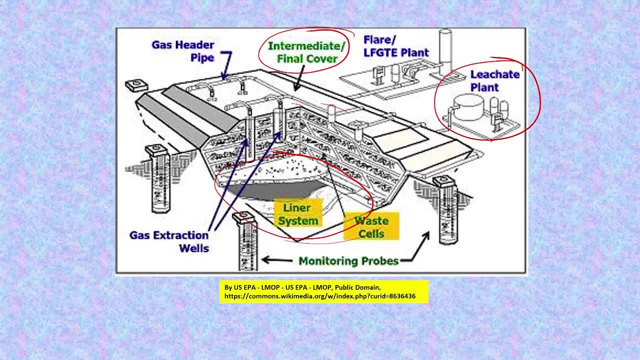 plant and then you can also collect the gas that is coming out of this landfill. You can extract the gas, use it for you know any useful purpose. This is in a simple terms. What is an engineered landfill is? and we also put all these monitoring probes or monitoring. 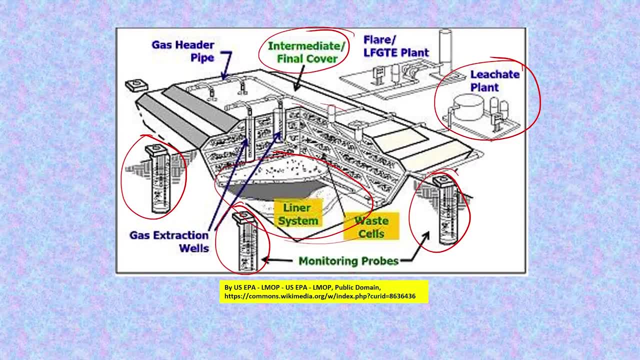 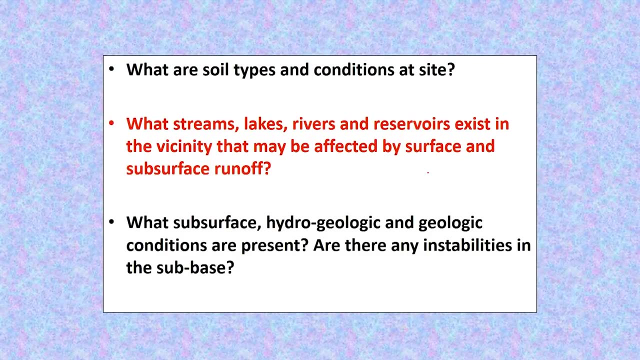 wells and we keep taking samples and then see whether the ground water, any leachate, is coming out of this landfill site. Now there are certain questions We have to ask. What are the soil types before we siting the landfill? 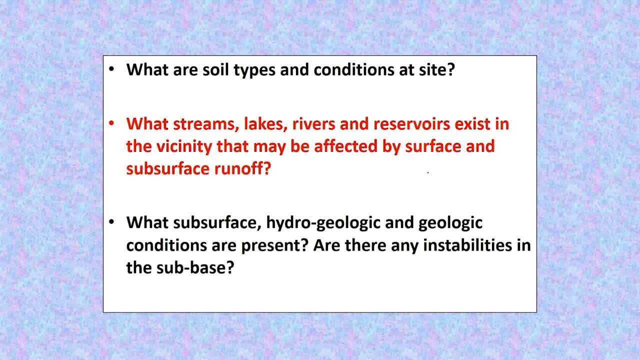 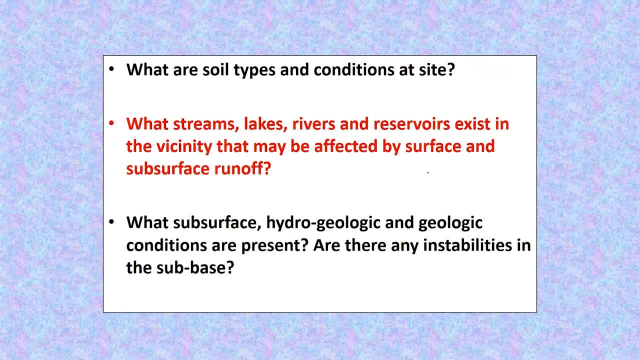 What hydro geologic? What hydro geologic? There are relevant questions about how do we know what types of everyday зависings 졠 are present? How do we know if traits, vegetables are present? How do if standards, forensic conditions are present? 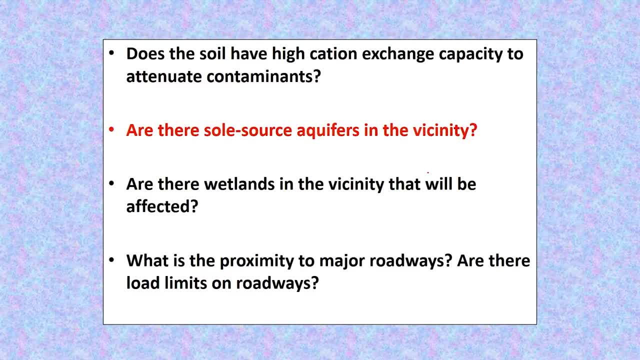 Are there any instabilities in the sub base? Does the soil have high cation exchange capacity to attenuate contaminants? Attenuate contaminants means as the contaminant moves through the unsaturated zone or saturated zone, its concentration keeps coming down. that is what we call attenuation. 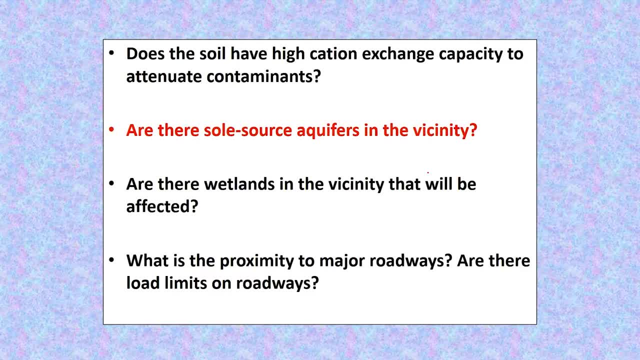 Are there sole source aquifers in the vicinity? That means if there is any source of water, either surface or subsurface, and that is the only source of water that you have, source of the water which can be, I mean the water from that source can be used for drinking after some treatment. So are there any soil sources in the nearby? are there wetlands in the vicinity that will be affected? what is the proximity to roadways? are there any load limits on roadways? aesthetic considerations: are there any airports in the vicinity? and the dump site may cause bird. 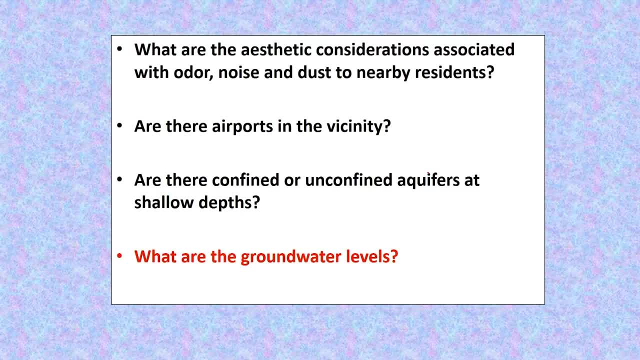 heads. are there confined and unconfined aquifers at shallow depths? because if the aquifer is at a shallow depth then the risk of contamination to the aquifer will be very high. What is the ground water level? Is the ground water level going to be above the surface? 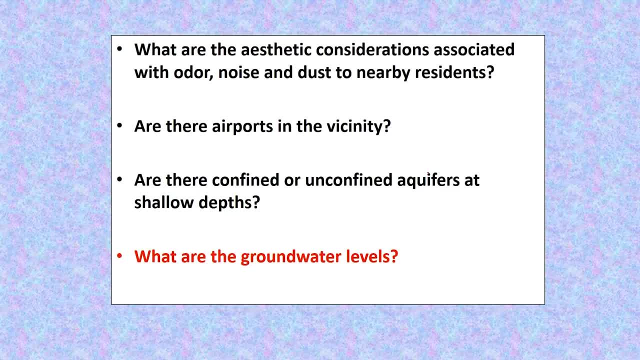 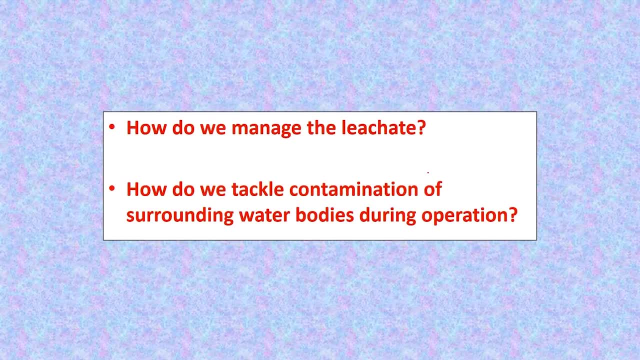 Above the base level of your landfill or it is very, very deep, and what are we doing to manage the leachate? whatever the leachate, it is contaminated with any high concentrations of hazardous chemicals. So how do we tackle contamination of surrounding water bodies during operation, like, for example, 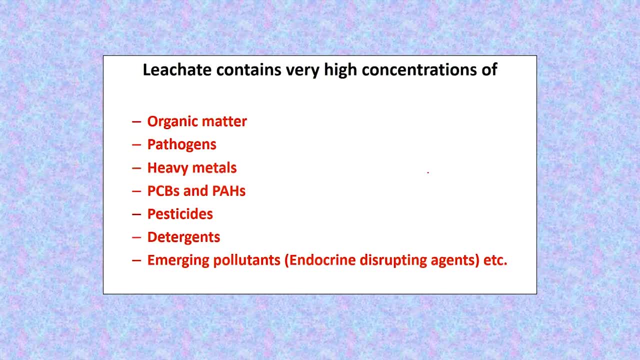 the leachate contains high concentrations: High concentrations of organic matter, pathogens, heavy metals, PCBs, PAHs, pesticides, detergents and emerging pollutants, etcetera. So what are we doing to manage this leachate? 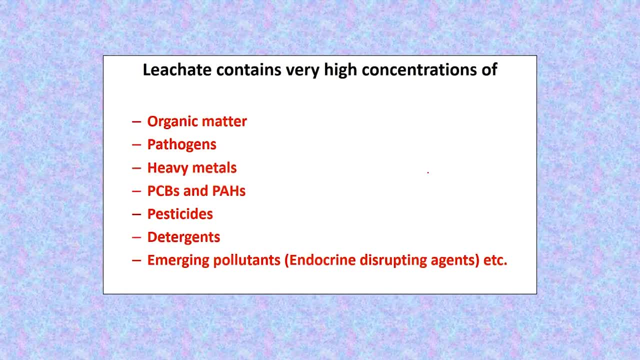 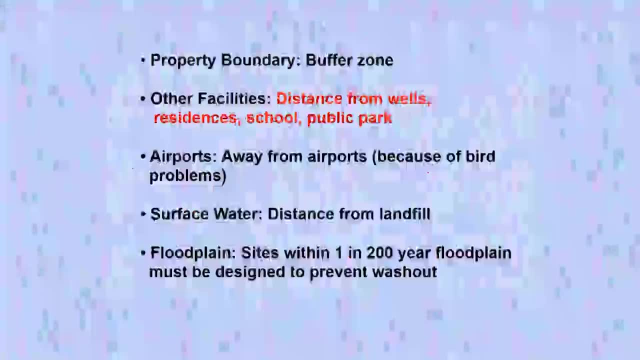 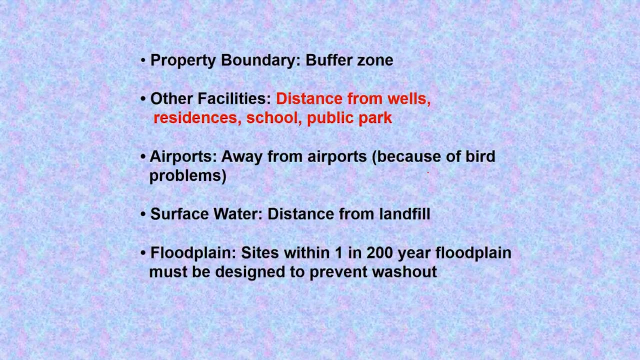 Are we collecting the leachate properly and treating it properly and then disposing it of? what is the leachate management that we have for the landfill? that is very important. Are there any property boundaries? Are we falling within the buffer zones? What are the other facilities? 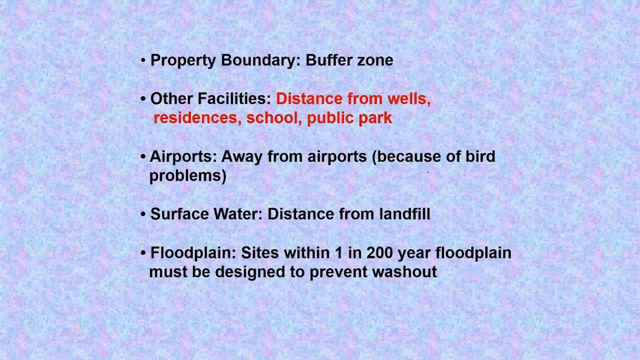 Distance from wells, residences, schools, public parks, then surface water. what is the distance from landfill to the river or tank or lake? Are we siting this landfill on flood plains? Are there any property boundaries? Are we falling within the buffer zones? 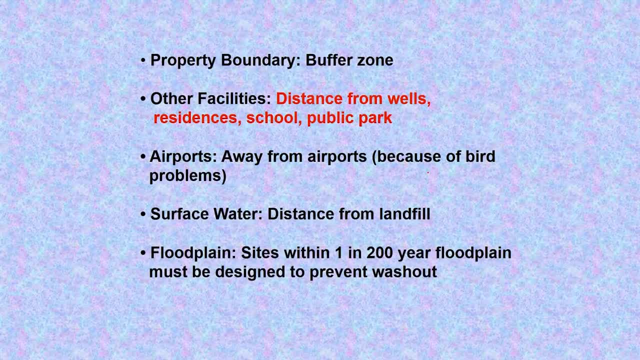 What are the other facilities? Are there any hospital facilities and facilities that can be getsvarious, And are we using systems or stations to start fight against these pursuits? Are there any facilities in the area? ofisiajwarded melting- not a source of residential water. 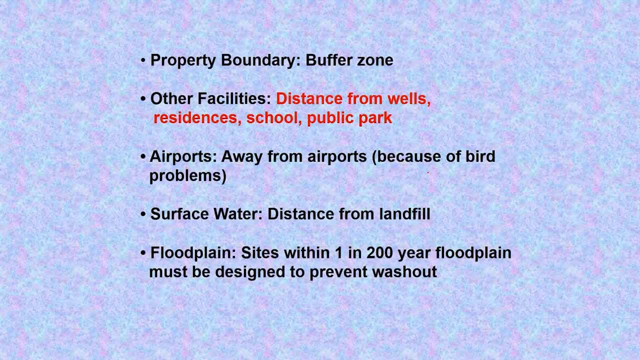 of daddy's waste materials. Is there anything that we will use there? Erasmus distillery resources like Urchins, sea셩, YTrace or Thermal dam settings to control that Got that. Is there water for children crying or safe pública water as well? 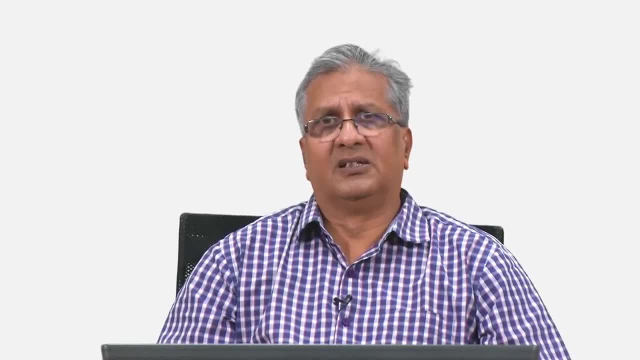 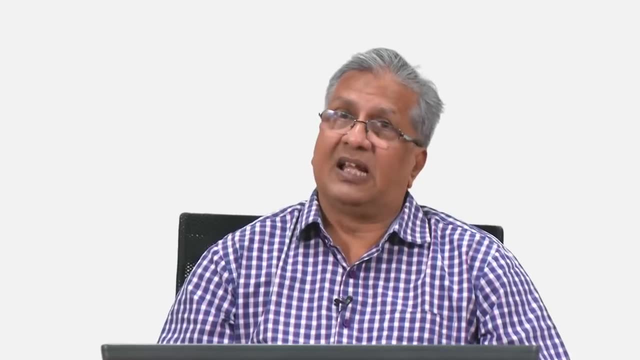 So all of these issues one needs to consider before we go and then do the siting of landfills. What will be the next steps for those parts? do the siting of landfill, but landfill itself is required very much as a part of our solid 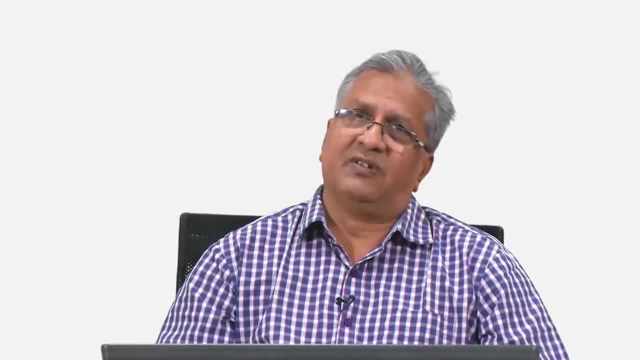 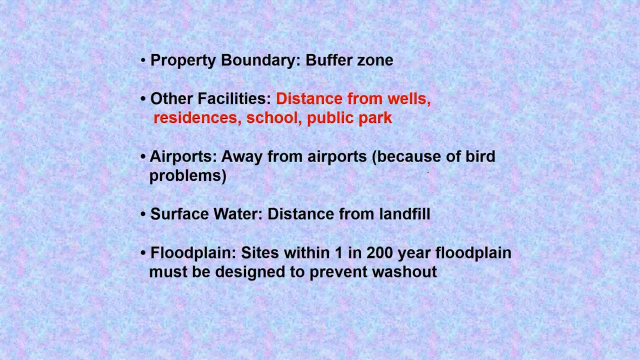 waste management. and if we do not do proper solid waste management then also we will be polluting our water sources. So you can see how all these issues are interconnected: Solid waste management, water resources management, public health, economy and, of course, the